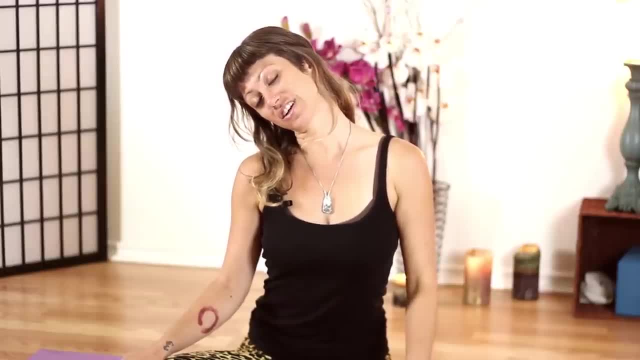 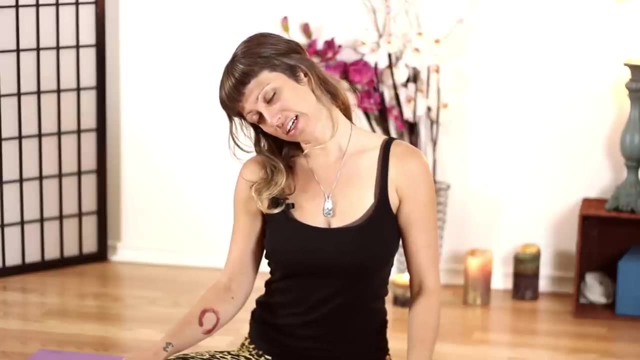 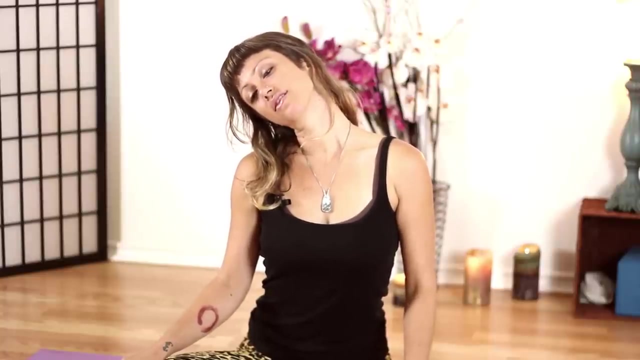 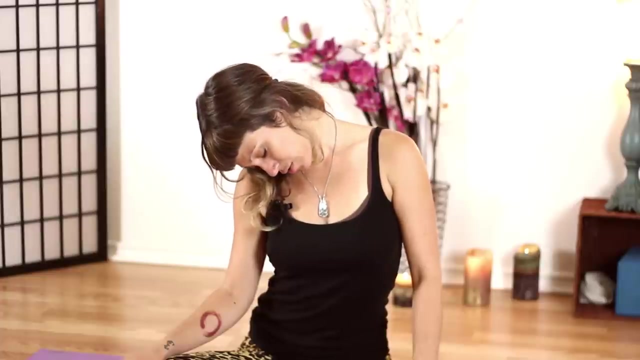 So just go ahead and breathe into that sensation. Take a big, full inhale and as you exhale, let your ear drop a little closer to your shoulder Again. take a nice big breath in and out. Now slowly roll your chin through center, rolling your chin down towards your chest. 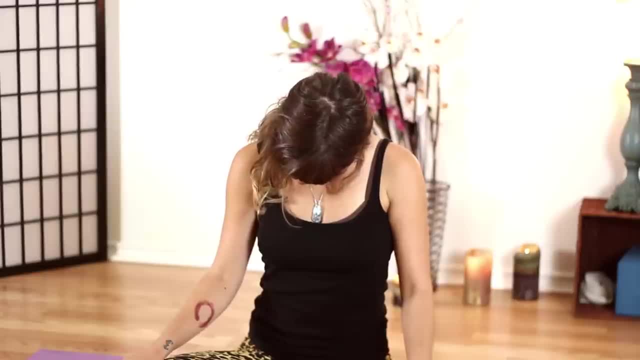 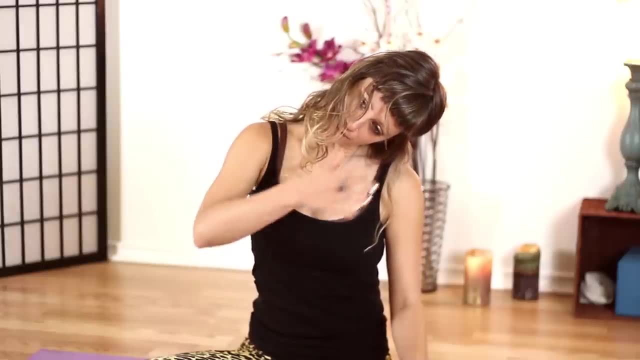 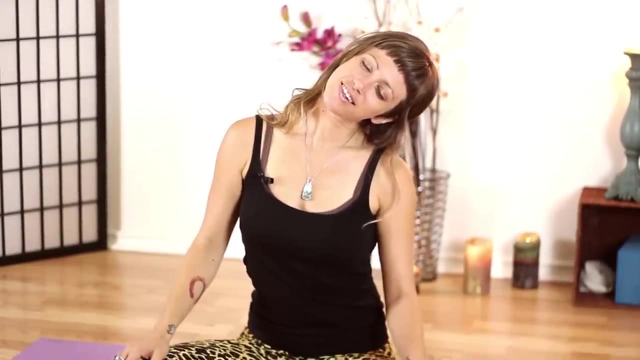 And continue this movement, rolling your head all the way across your chest until your left ear comes towards your left shoulder. So now you're stretching across the right side of your neck just breathing into that sensation. So again here, let's take a couple of nice deep breaths, Take a full inhale. 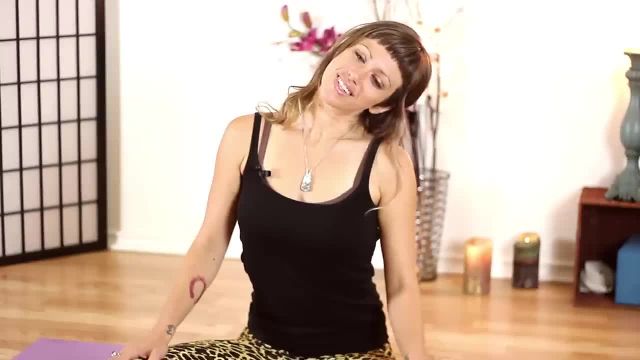 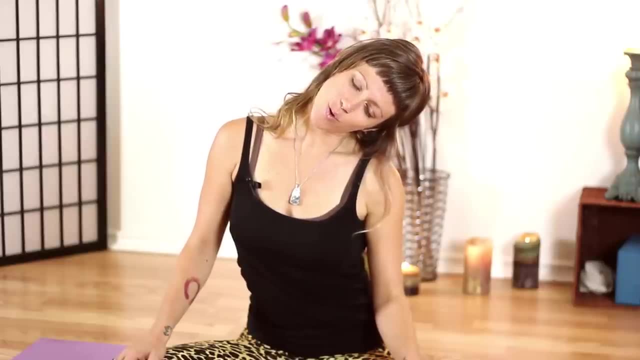 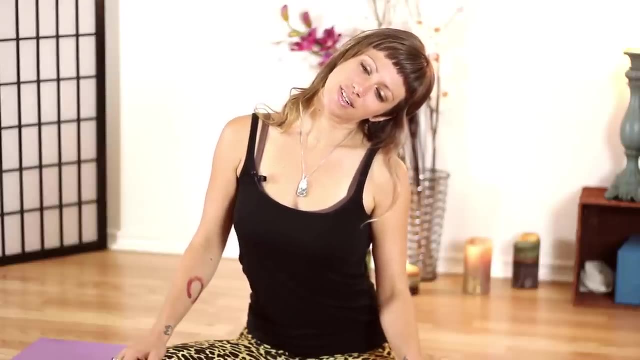 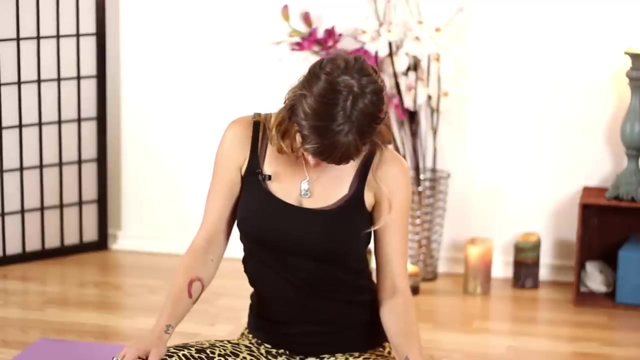 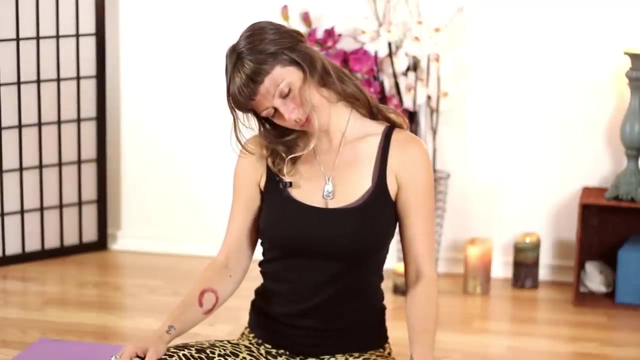 And as you exhale, let your head relax a little bit more. We'll go one more time. Take a big breath in and out And again, slowly roll your head through center, rolling your chin down towards your chest And all the way across to the right side. 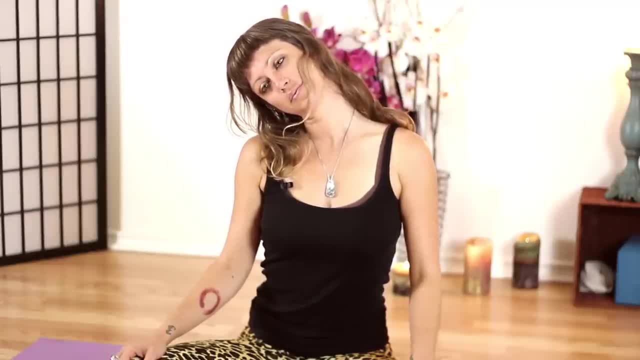 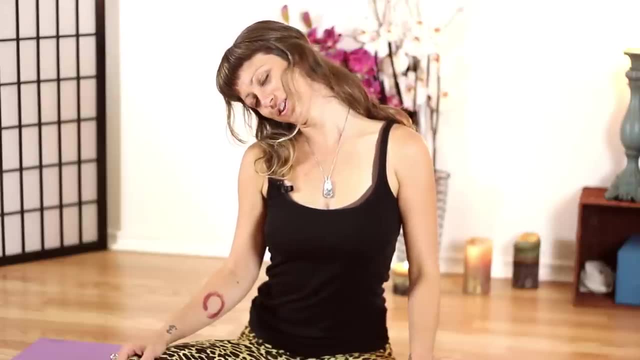 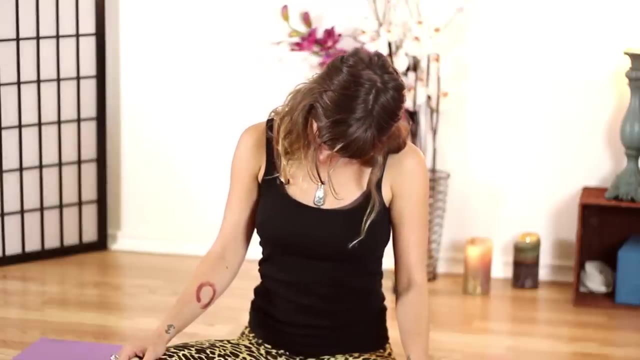 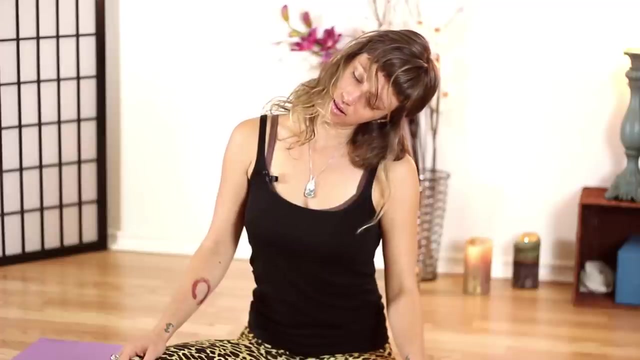 Take a full inhale once you arrive And a full exhale. Take a deep breath in and out And a full exhale And then roll your chin over to the left. You can go nice and slow, Really feel every bit of sensation as you stretch across your neck and even through your spine. 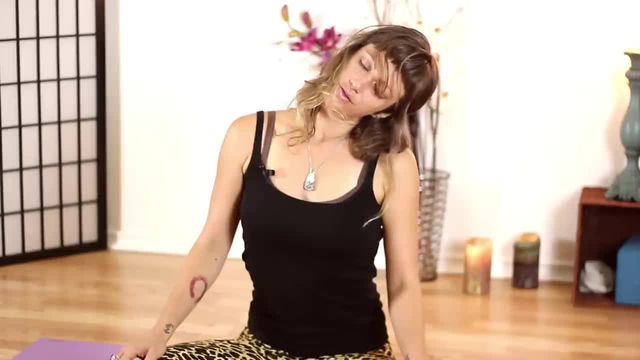 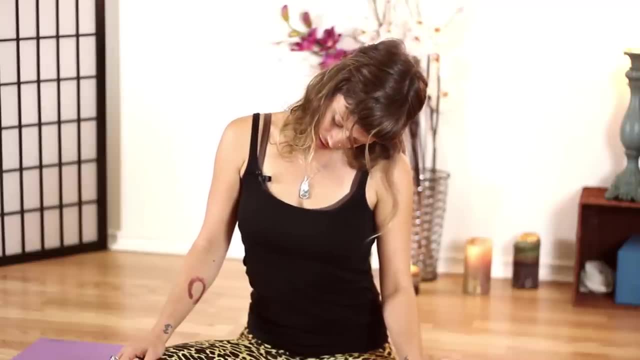 Take a big breath in And out And we'll go one more time to both sides. So slowly roll your chin through center and over to the right, Take a full cycle of breath. And roll your head over to the other side. Take a full cycle of breath. 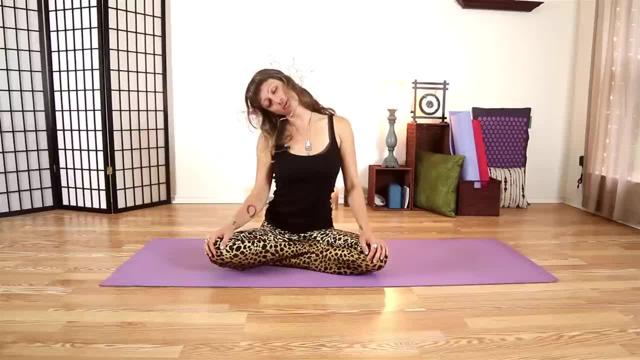 And roll your head over to the other side. Take a full cycle of breath And roll your head over to the other side. And roll your head over to the other side. Take a full cycle of breath And roll your head over to the other side. 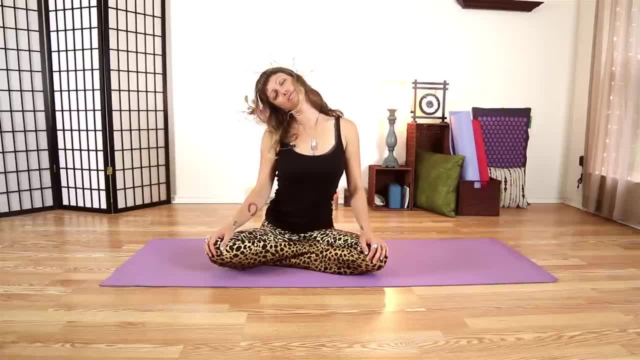 Take a full cycle of breath And roll your head over to the other side And roll your head over to the other side. Take a full cycle of breath And roll your head over to the other side And roll your head over to the other side. 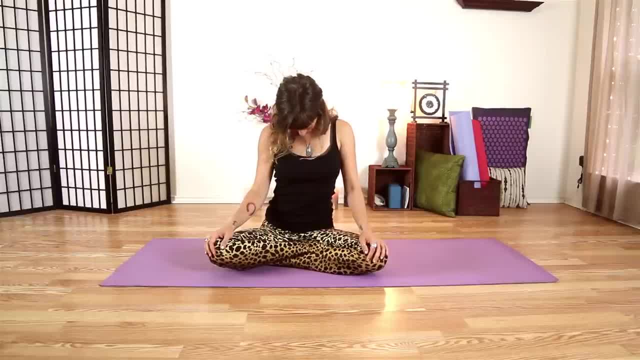 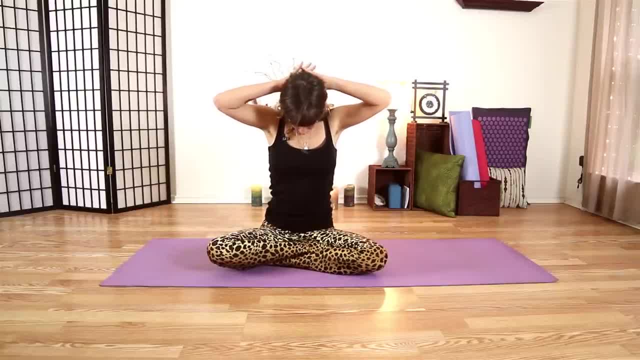 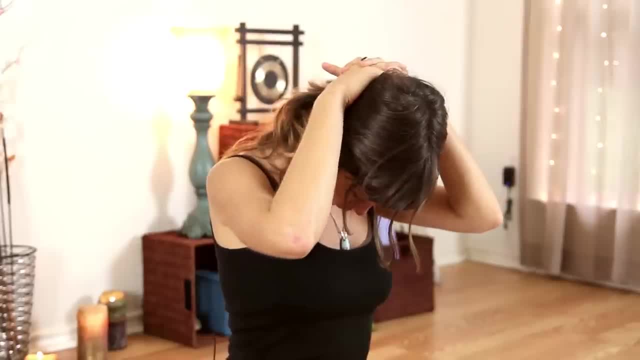 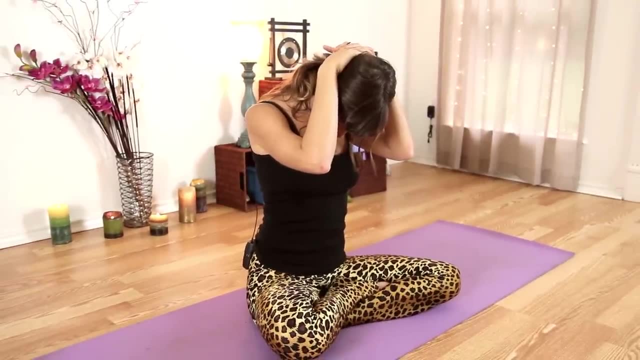 Interlace your hands at the back of your head- so not so much behind your neck but really at the back of your head- and let your elbows drop down towards the floor, so the weight of your arms provide a little traction for you as you gently stretch the back of your. 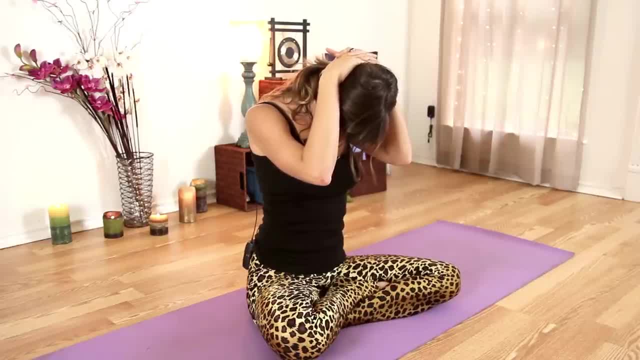 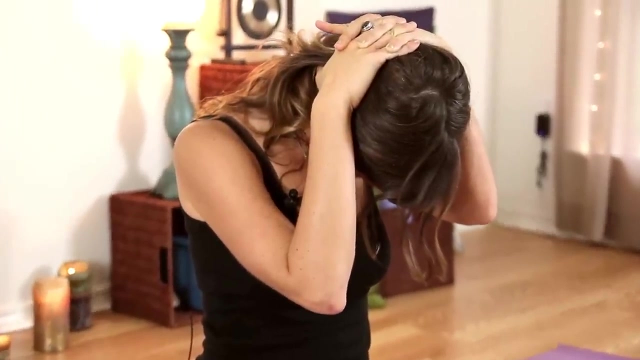 neck. You may even start to feel some sensation stretching down through your spine. Then, gently and slowly, just turn your head a little towards the right and to the left, a little at a time, and keep drawing your chin down towards your chest so as you slowly roll. 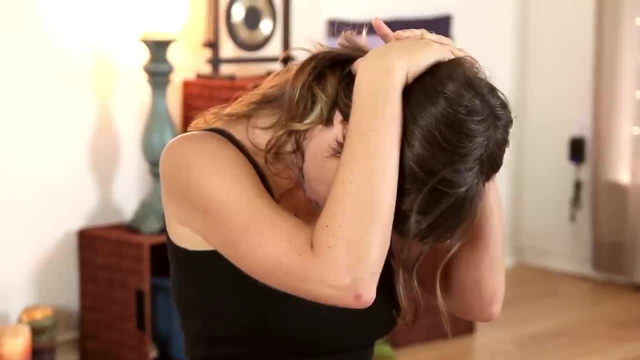 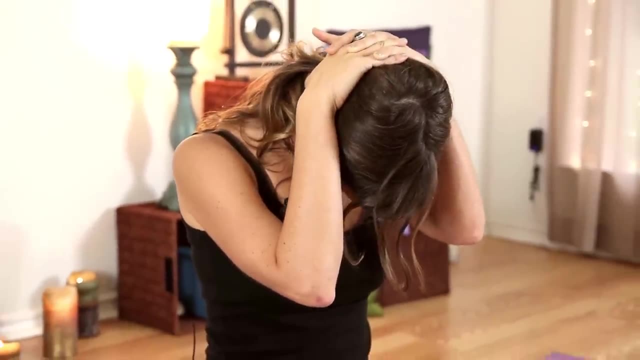 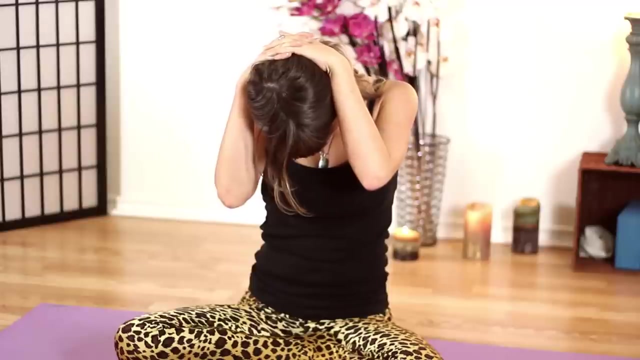 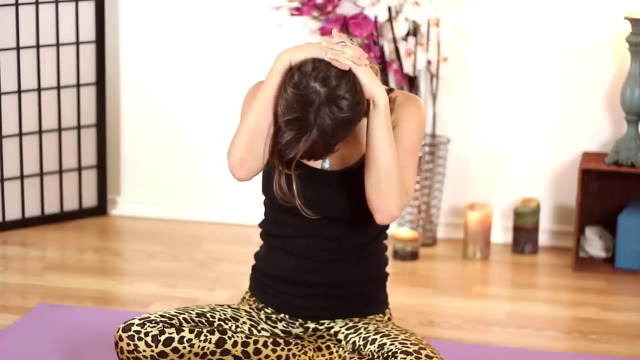 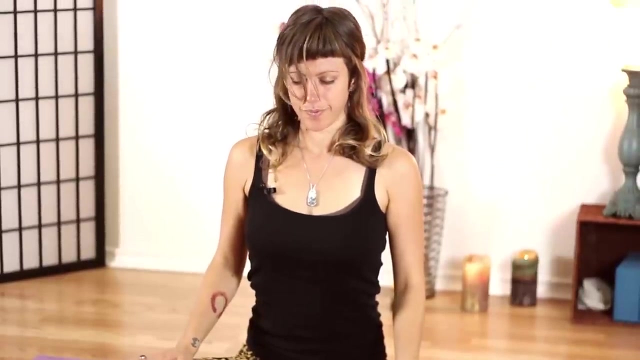 your head right to left. you're going to feel this stretch kind of shifting from one side of your back to the other, And gently make your way back to center, Release your hands and let your head slowly roll up. All right, So that's it. 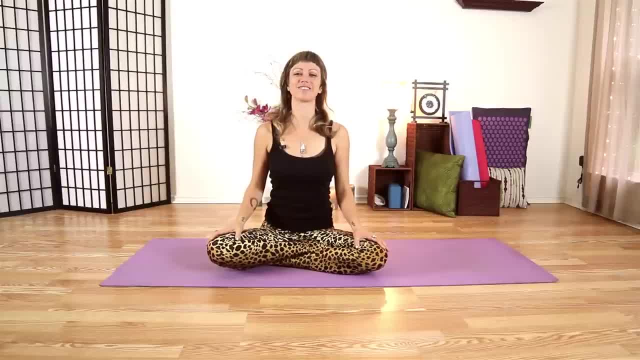 Good, Good. So now that your head and neck is feeling a little more loose, let's just make some full circles, rolling your head all the way around. Try not to crunch your neck when you roll your head to the back, but rather think about. 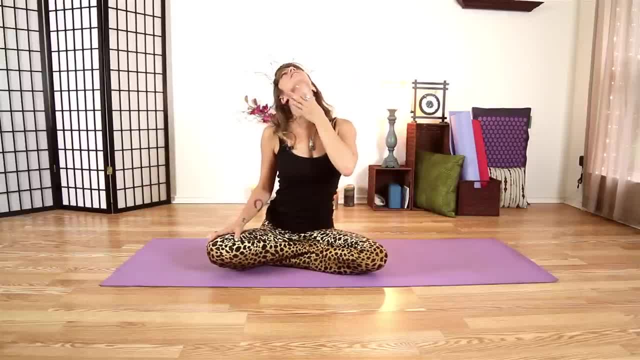 lifting your chin towards the ceiling. That's going to help you stretch the front of your neck without crunching the vertebra at the back of your neck. Good, Good, Good, Good. And after you've made some circles going one direction, let's reverse and make a few. 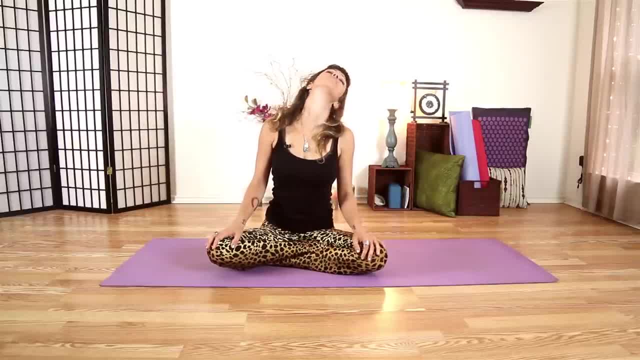 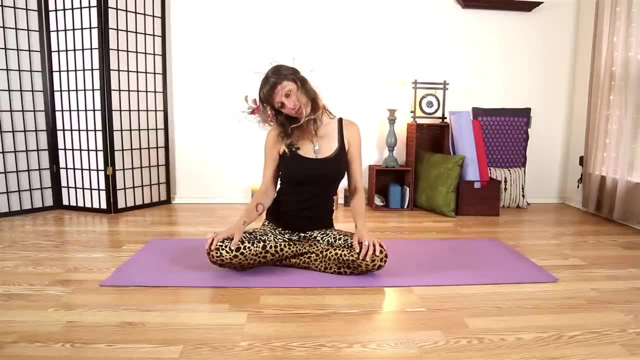 head circles in the opposite direction And just pay attention and notice any places where your neck feels tight, where it gets a little stuck, feels a little pinchy Good. So these are areas that need to be stretched. so you're just noticing what's happening in. 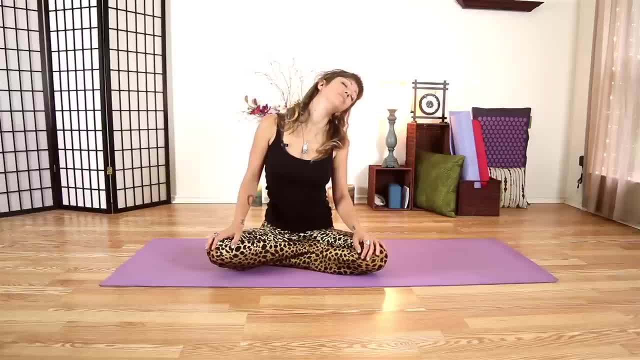 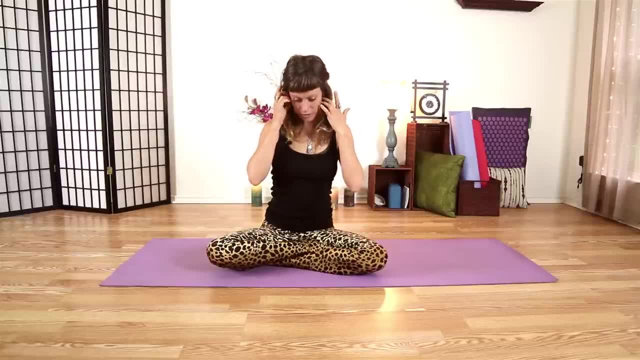 your body And after you've made a few circles in the other direction, then we'll come right back up to center. So now we're going to start doing some things to stretch into your shoulders. so start by drawing your right arm across your chest. 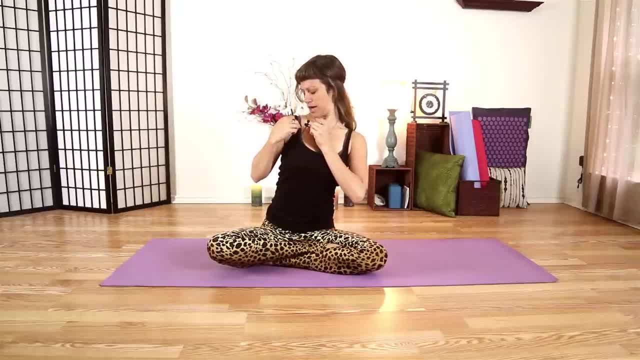 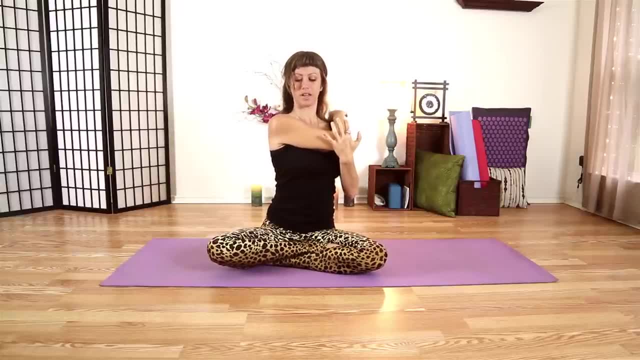 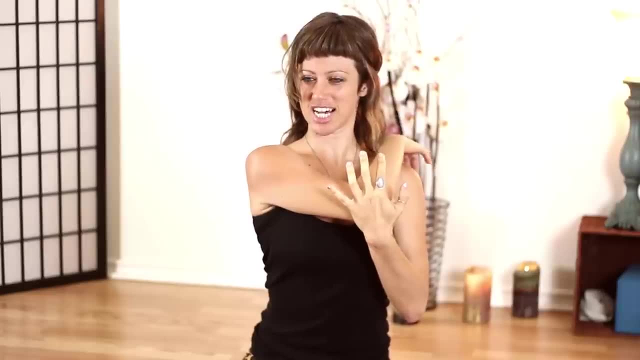 I might lose my microphone here. let's see if I can move that up. You can draw your right arm across your chest, stretching into your shoulders. It's like giving yourself a big hug. as you draw your arm across your chest, I'm using my left hand to press my elbow. 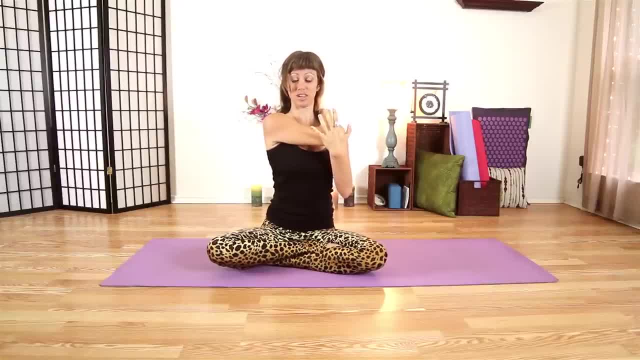 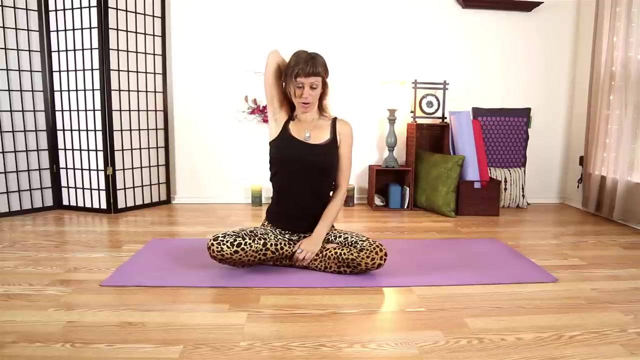 This is helping me get a nice stretch, Stretch across the backs of my shoulders- and I'm even feeling a little stretch kind of between my shoulder blades there as well- and release and then lift your right arm up towards the sky, drop your hand down between your shoulders and you'll reach your left. 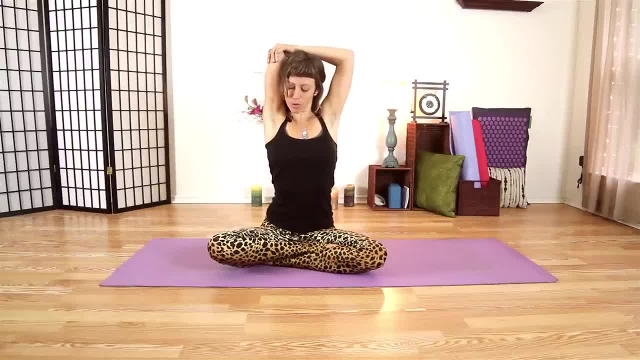 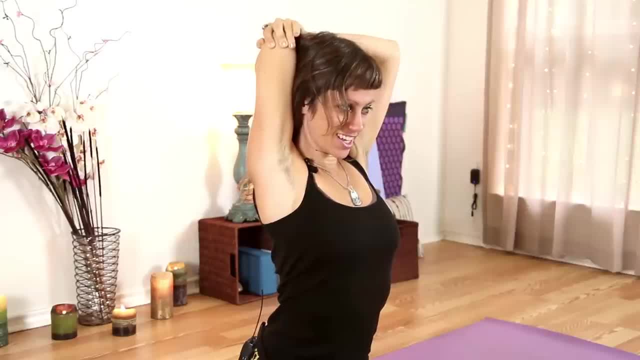 arm up, Grab a hold of your right elbow And pull back towards the back of the room. This is going to help you stretch along your shoulder and into your triceps as well. So keep lifting through your spine, lift through your chest and draw your right elbow back. 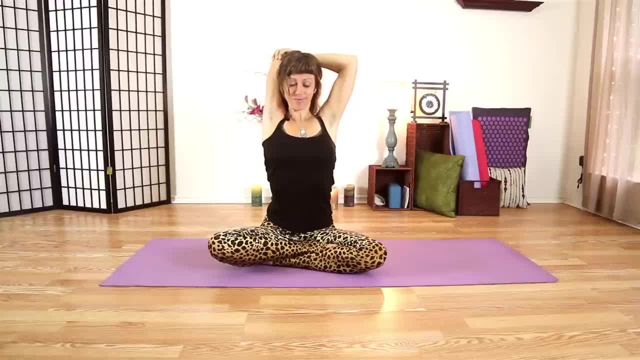 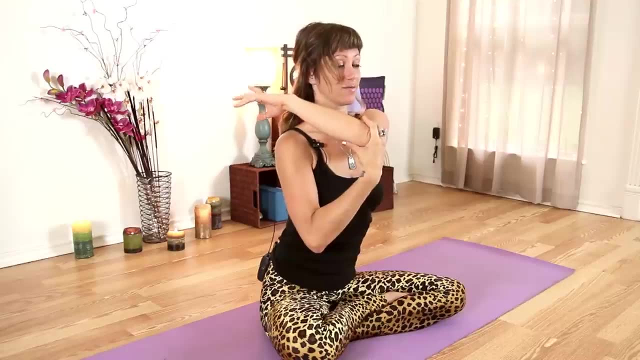 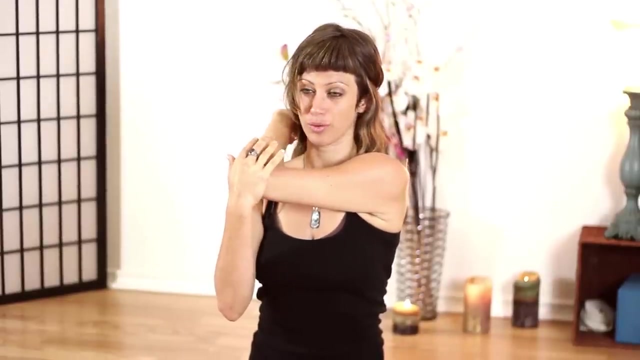 behind you And gently release Good Good, Good, Good, Good Good To the other side. bring your left arm across your body, Use your right hand to really press your elbow across your chest. Just enjoy the sensations that you're feeling. 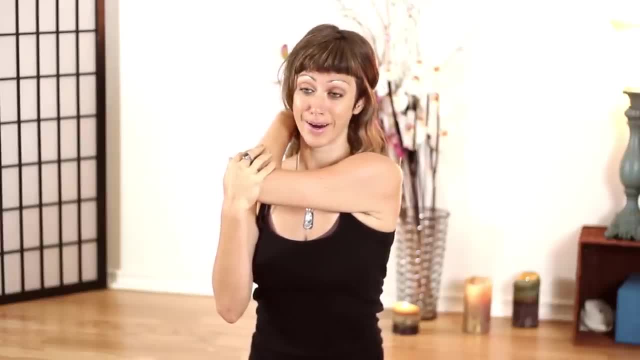 Wherever you're noticing that stretched sensation is where your muscles are tight, So that's where you need it. That's where it's holding tension. So we really want that. You really want to just breathe into those places. Take your time. 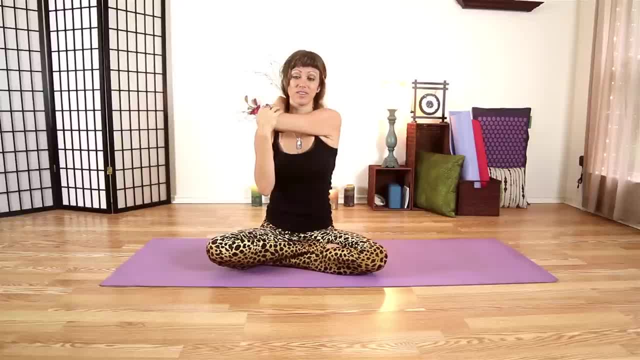 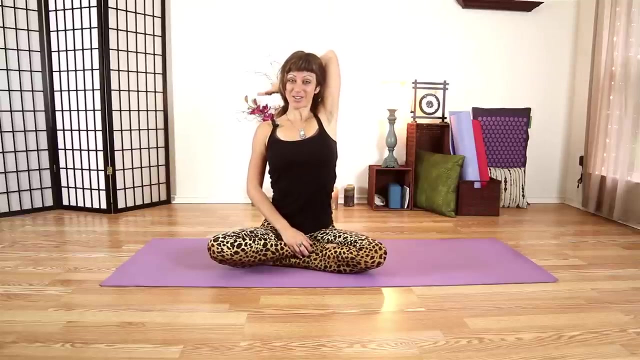 Be gentle and compassionate with yourself And invite those muscles to relax and open up, increasing that flexibility and mobility, And we'll release the stretch And reach your left arm up. Bend your elbow and let it drop down behind your neck. Take your right hand to grab your left elbow. 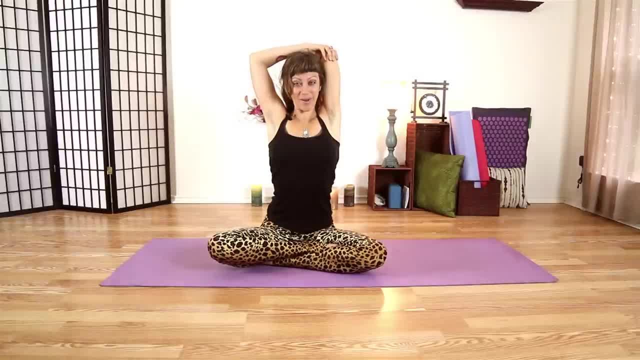 and help it out. You want to stretch it back behind you. Keep lifting through your spine, lifting through your chest. This will help increase the stretch sensation And remember we're breathing all the time, Breathing into every little tight place in your body. 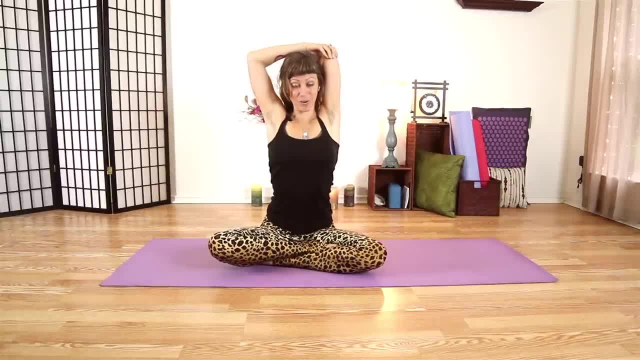 Your breath is the key. That's what's going to help you release that tension. So, when we get into stretches that feel challenging, the tendency is to want to hold your breath until it's over, But the trick is to keep breathing. That's what's going to help you relax. 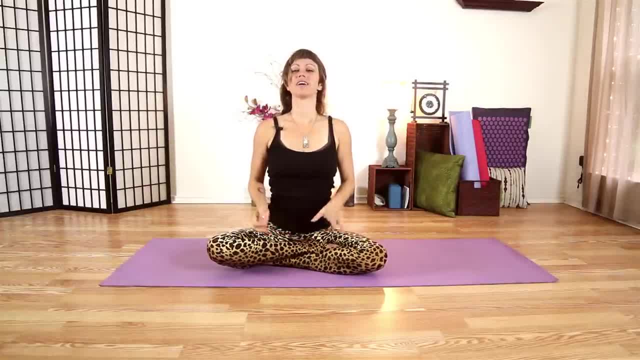 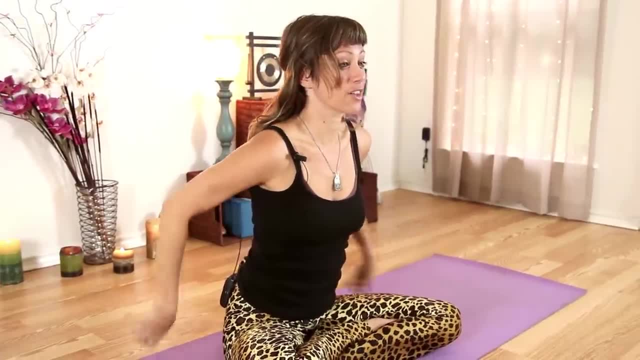 So we'll release that shoulder stretch here And this time interlace your hands at the back of your spine, Squeeze the palms of your hands together So it's like you're holding your hands. You're saying grace, You're going to squeeze your hands together really tight. 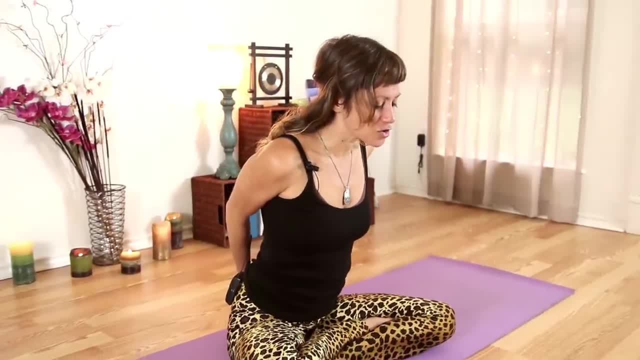 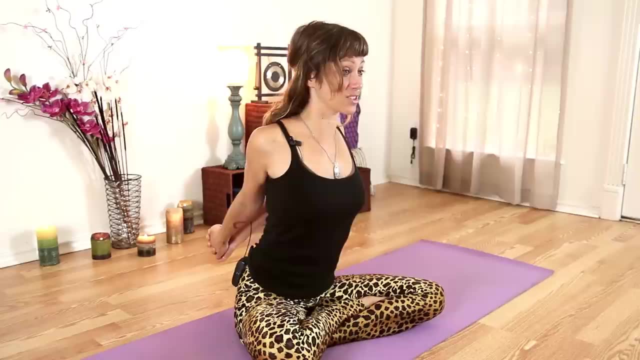 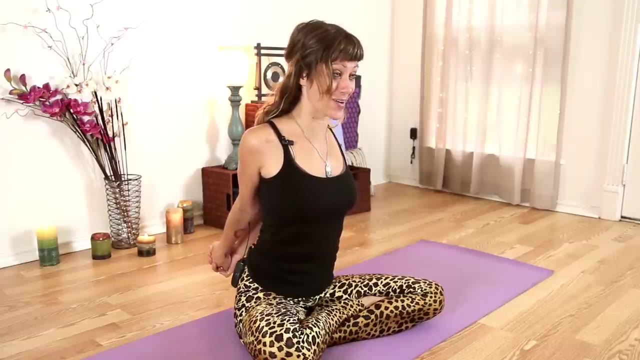 at the back of your spine, Then stretch your fists away from you towards the wall behind you, Reach your hands back as far away from your hips as you can. So for some of you with really tight shoulders this is going to be challenging, I know. 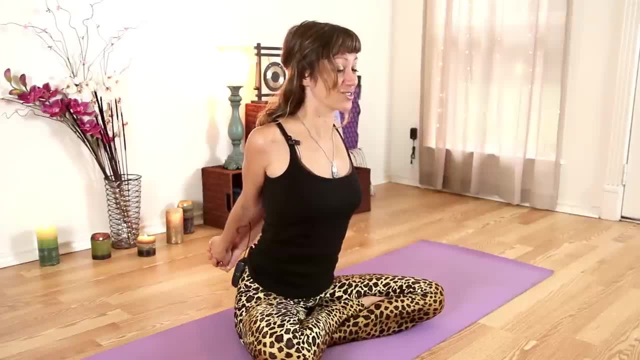 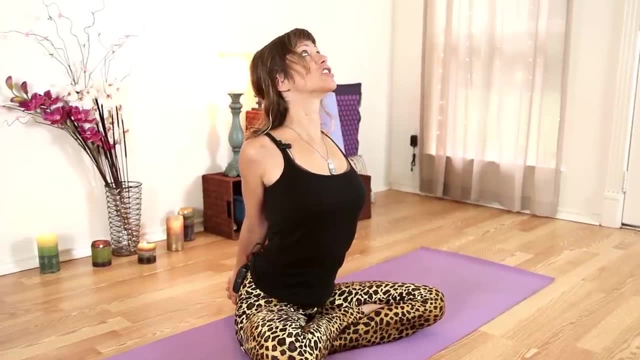 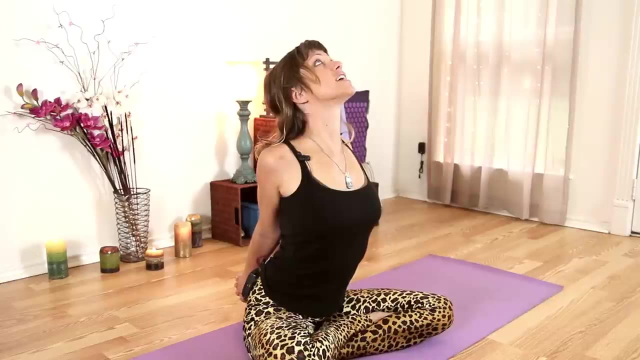 But accept that, Accept the challenge. You can do it. Stretch your fists as far away as you can And then start to lift your heart up, opening through your chest. So a lot of times when we spend time sitting at the desk, 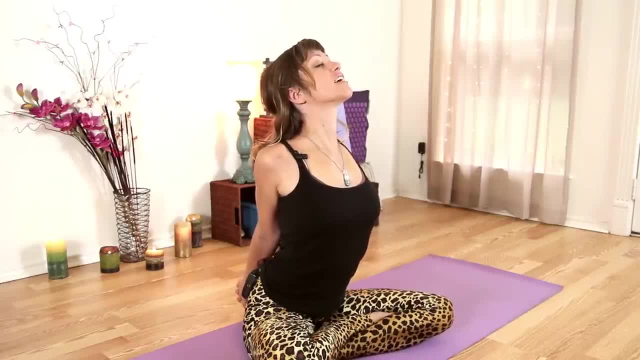 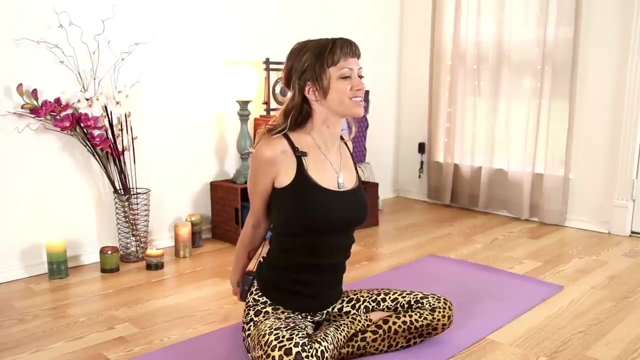 working at the computer, our chest gets tight, really tight and rounded. So this is your moment to reverse that pattern. Open your chest, Open your shoulders- You can even lift your gaze and open your throat- And then we'll slowly return back to center. 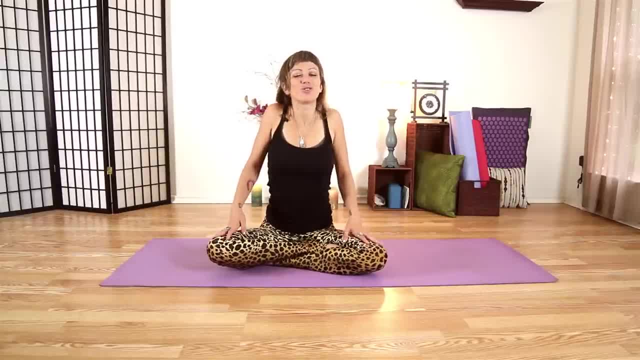 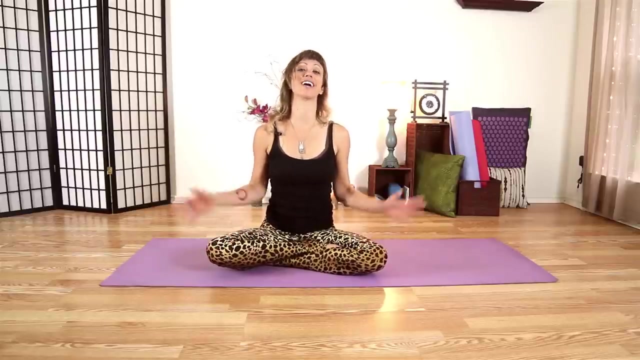 All right. So just make some circles with your shoulders circling up towards your ears and back behind you And reverse directions, And that must be chest stretch, All right. So we're gonna do one more really nice little chest stretch before we wind down our practice and take a moment to rest. 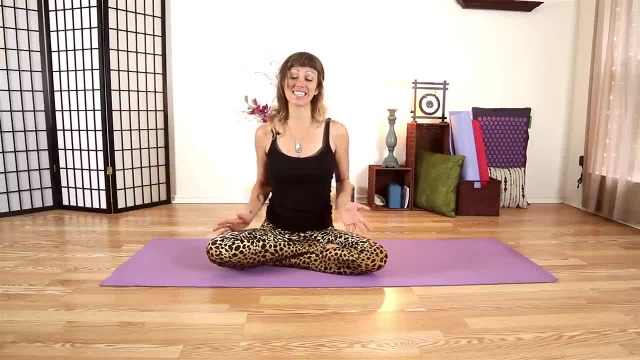 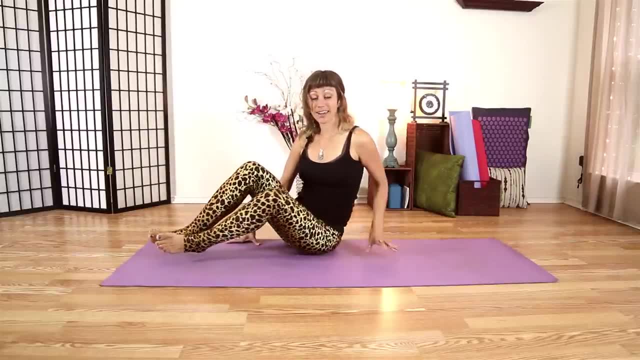 So if you are sitting in a chair, I recommend that you go ahead and make your way down onto the floor, if you can. If you're already seating on the floor, then go ahead and lay down my left side, but it really doesn't matter, we're going to do both, so lay onto your side. 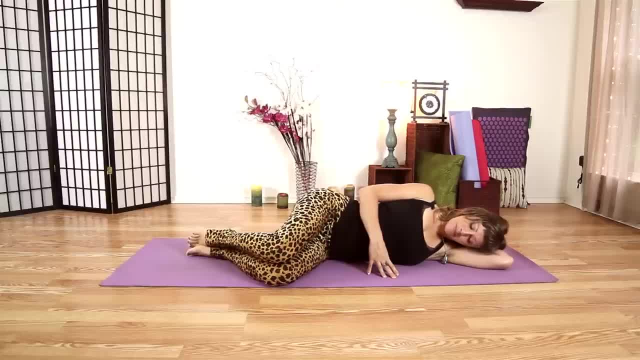 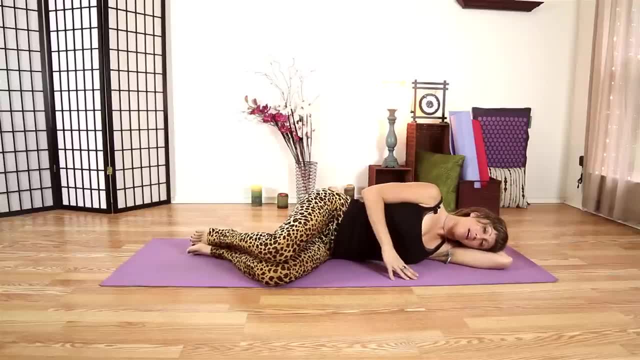 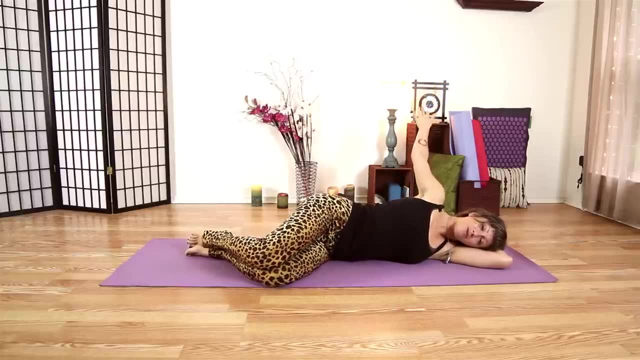 you can support your head with your arm that's underneath, and the goal here is to keep your shoulders stacking, so you don't want to roll your chest open, but keep laying completely on your side and sweep your right arm up and around so you reach your right fingertips towards the back. 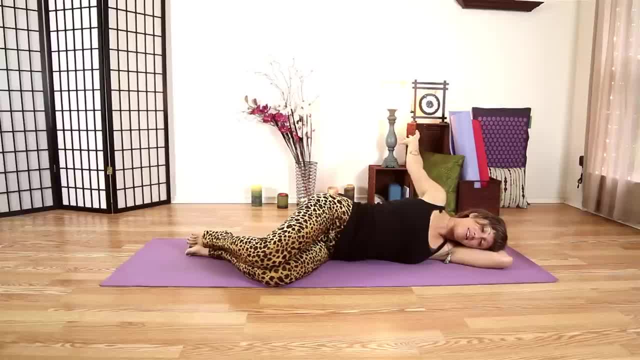 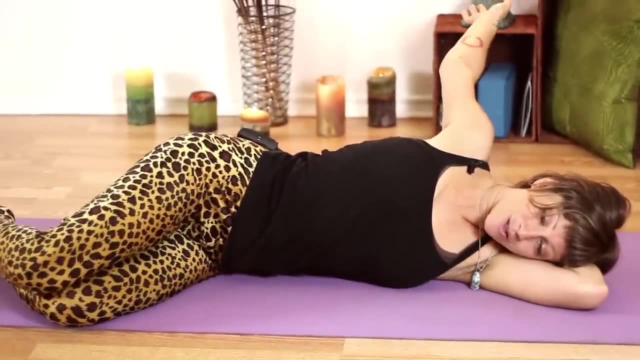 wall behind you so you can see that if your chest is tight, your shoulders want to open up to the side, but remember to keep your shoulders stacking one on top of the other and then gravity is going to do the work for you, stretching your chest and shoulders, releasing that tension. 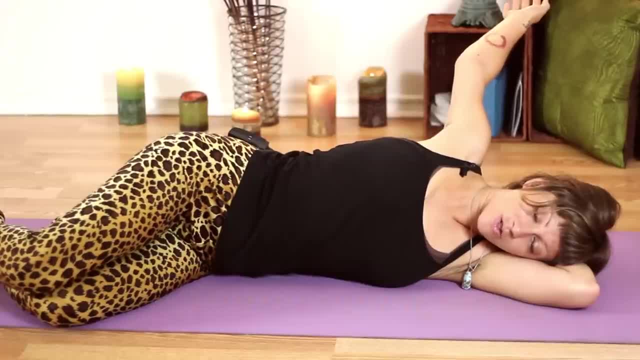 and so, as you stay here, you can find where's that sweet joy that you're feeling right now, and then you're going to take a deep breath and you're going to take a deep breath, and you're going to take a deep breath and you're going to take a deep breath. 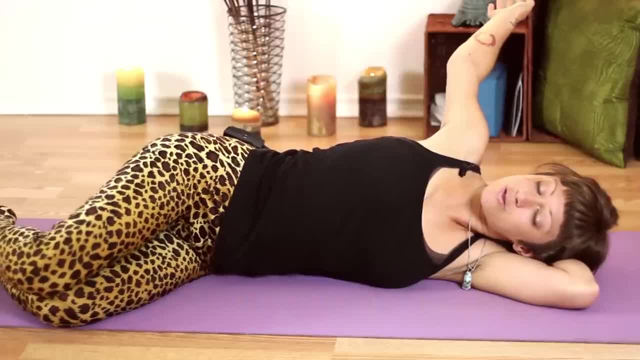 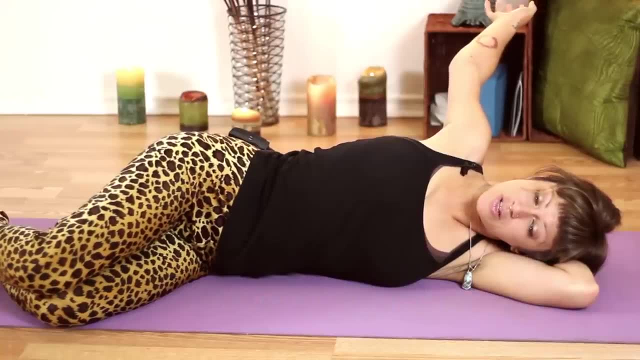 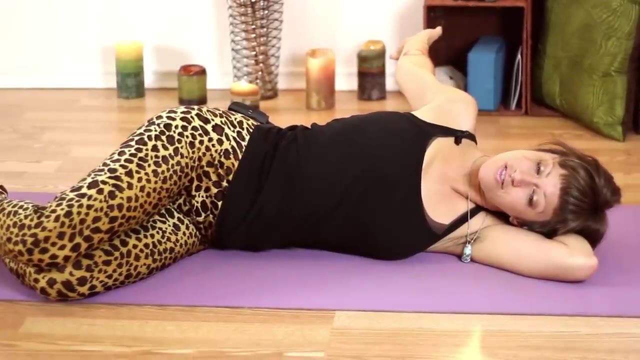 maybe staying in the right place, but if you feel you're in a juicy spot, wherever it's super tight, you can spend as much time as you need stretching into that area and as you explore the range of motion, you can sweep your fingertips down a little closer to. 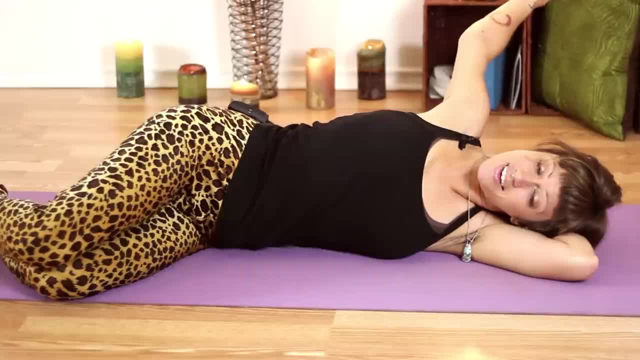 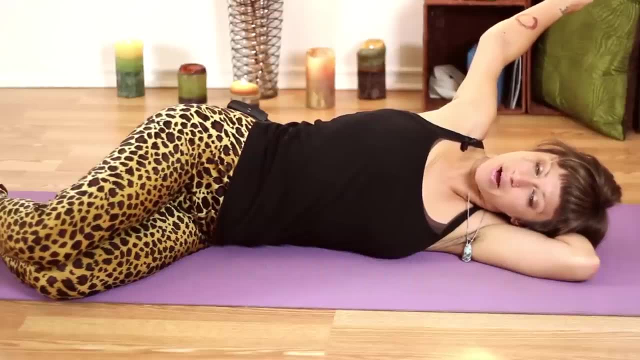 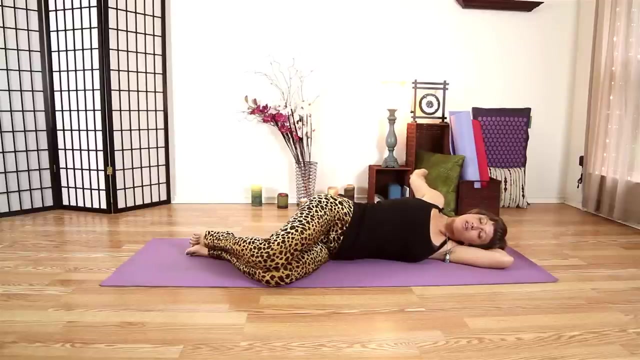 your hips, that will change the stretch. or you can sweep your fingertips up a little closer towards all along your chest, so you can just explore that range of motion, find where the stretch feels the best for you and we'll just stay with it, enjoying the sensation and staying with your breath. so I really like this chest stretch. so 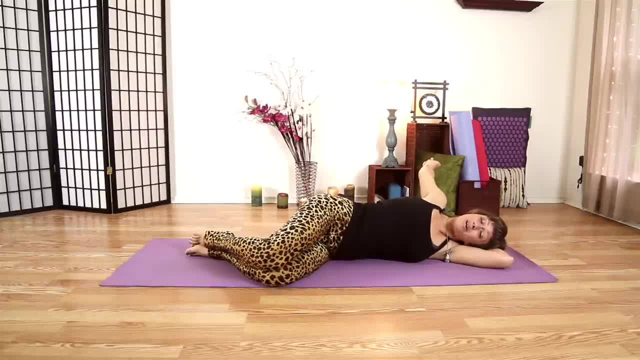 easy to do. you can do this in bed in the morning before you wake up or even before you go to sleep. this is perfect. or if you're watching your favorite TV show, you can just lay right there, watch something while you let your arms and chest and shoulders stretch. so it's really nice to be able to have something. 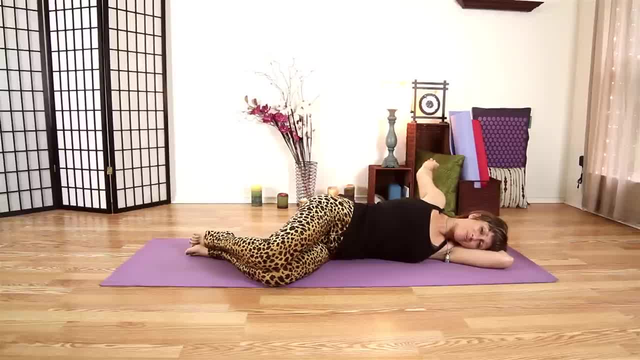 so simple that you can do. that's so beneficial. you can just let your right arm or your top arm gently come down by your side, just feel that sensation of your shoulder being stretched out, and then you can roll over onto the other side. so I'm just gonna flip over here, so I can. 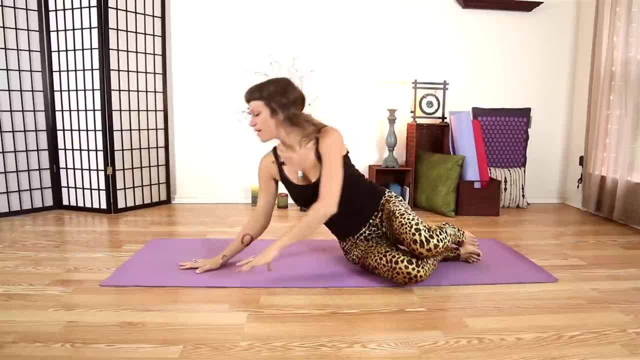 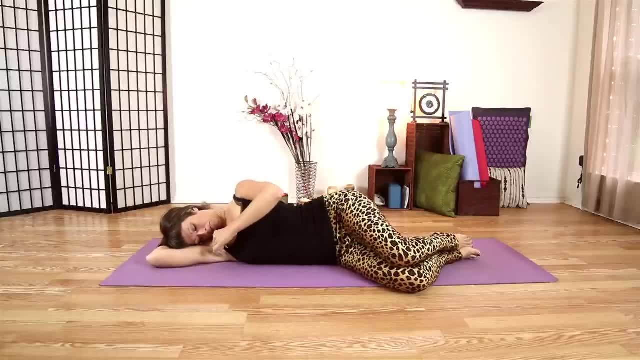 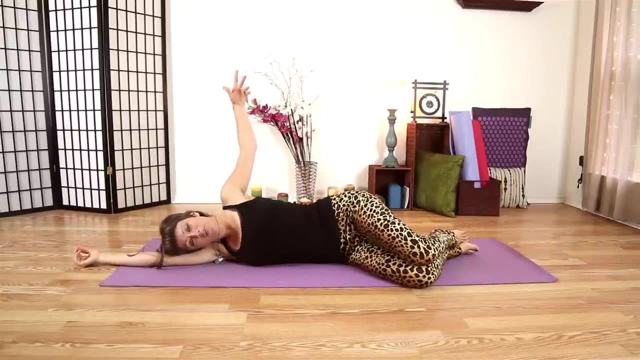 still face you and again you can use your hand to support your head and then let your top arm reach up and back behind you. keep your shoulders stacking right, so I'm gonna keep your body right in line as you let your other arm drop down behind you, slowly start to relax and you may. 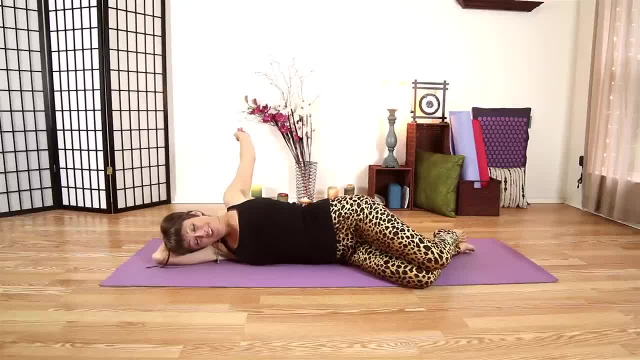 notice that one side is more tight than the other. it's perfectly normal. we rarely hold tension the same on both sides. you know it varies. so just whatever you're noticing, just observe that and be a witness. you don't have to change anything or do anything to. 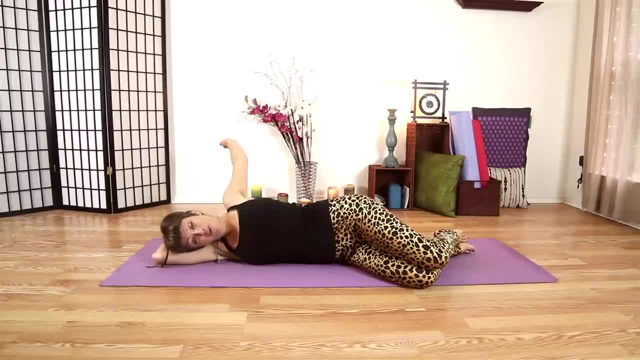 fix it and just let gravity do the work, slowly and gently, letting your chest and shoulders open. and again you have the option to extend your fingers a little closer towards your hips or your feet and feel how that changes the stretch for you, or you can extend your hand a little more. 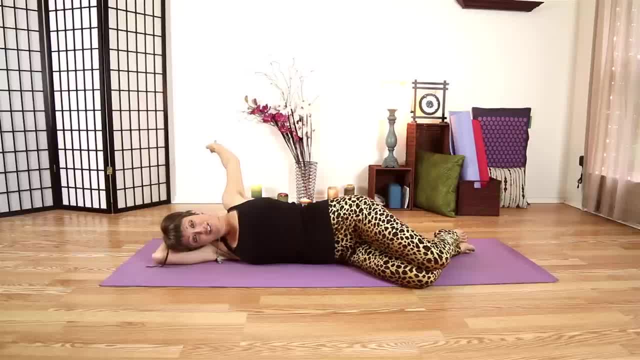 towards your head and feel how that changes the stretch. so you just find that spot that supports you the most. you'll stay here for another few cycles of breath, so I hope you're staying connected with your inhale and your exhale. your deep, relaxed breath helps your body to relax and release tension. 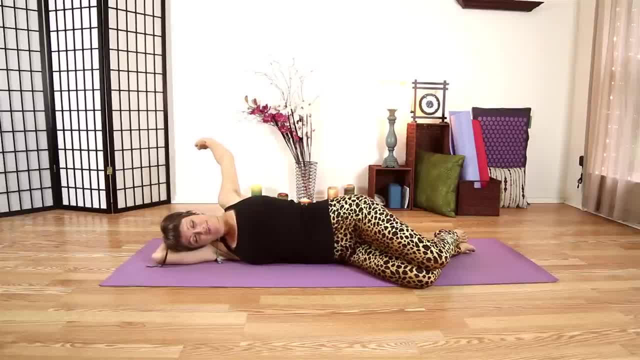 so we'll just take another moment here and, as you're ready, whenever you feel balanced, just let your left arm go, come all the way down alongside your body and feel that sensation of your shoulders stretched out and go ahead and just lie onto your back from here. 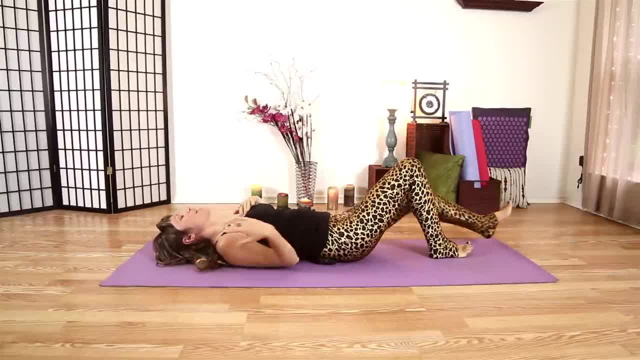 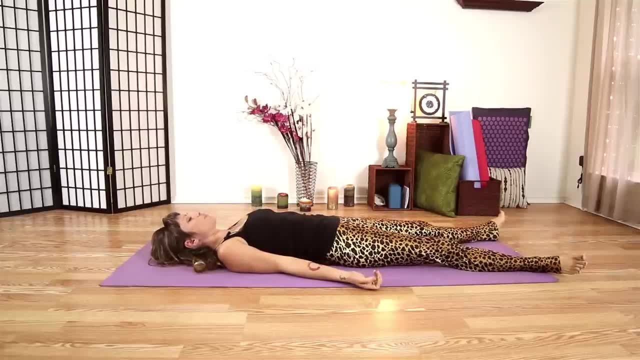 to just roll onto your back and take a moment to let yourself relax. let your breathing be deep and fluid and let your palms rotate up towards the sky, feel your breath moving in and out of your body and feel your chest and shoulders open and relaxed. you can gently roll your head from side to side and just relax. 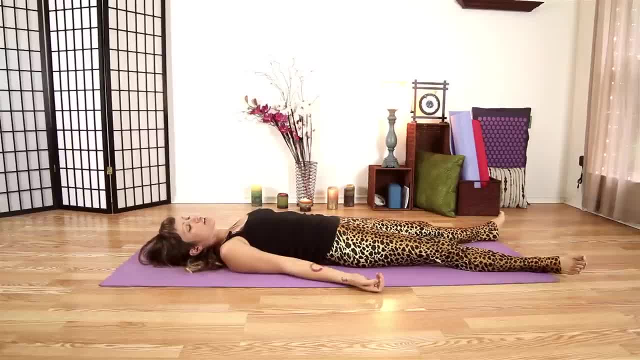 and, as you're ready, find your way to stillness. you can think of this as a little bit of a timeout before you walk away. just let that breath flow into your body and do that as a little exercise and just relax. and then, as you're ready, 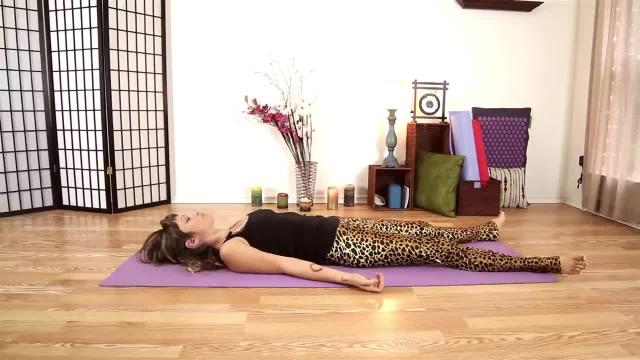 find your way to stillness, to just enjoy this moment of relaxation and relax, and relax and relax, and you're welcome to stay here and enjoy this time to rest for as long as you need and as long as you have time for and whenever you're ready to come out of it. 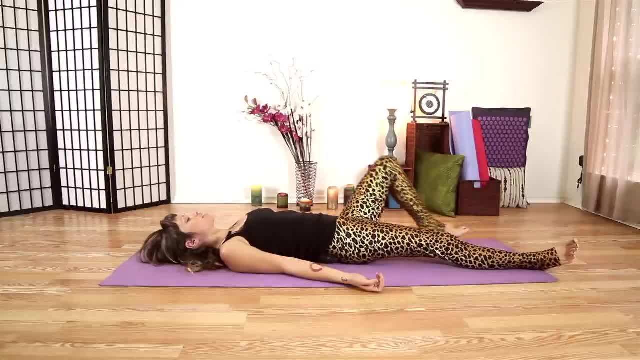 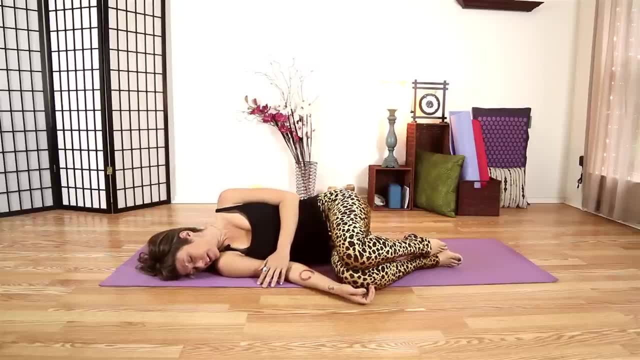 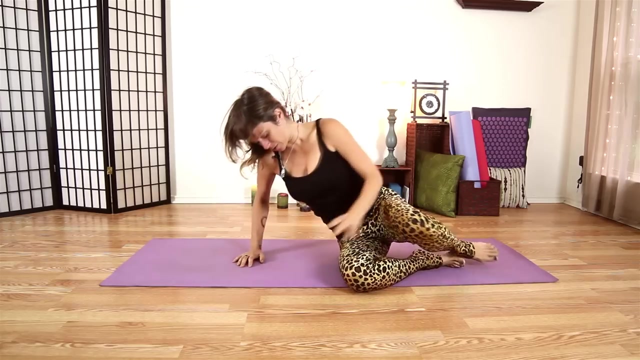 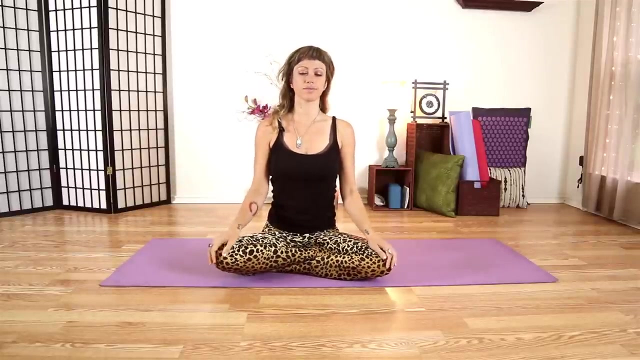 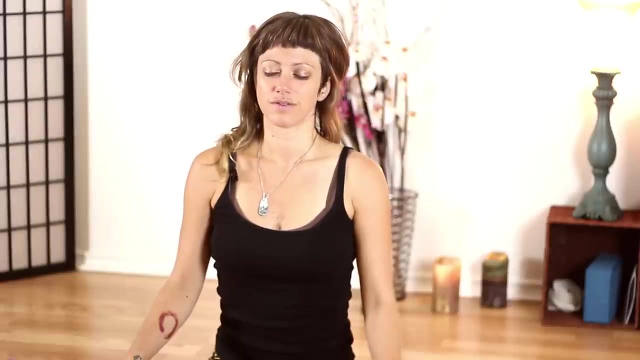 gently roll over onto one side, taking time to pause in a comfortable feet position, just letting yourself relax and slowly press yourself all the way up, coming back to a comfortable seat and just take a couple of nice deep, full breaths here and take this moment to acknowledge yourself. 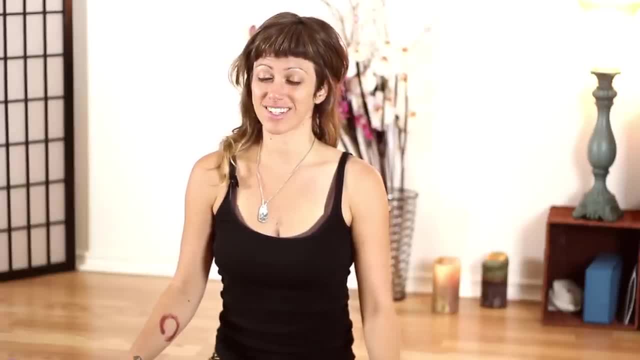 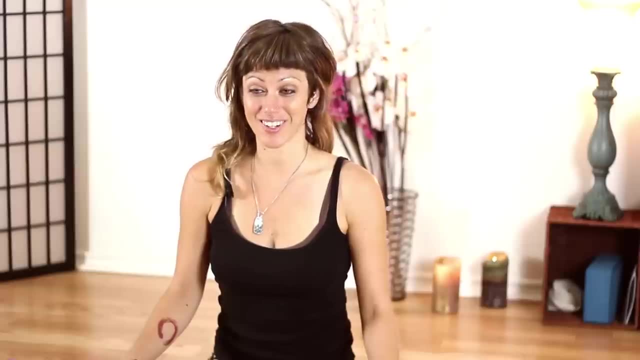 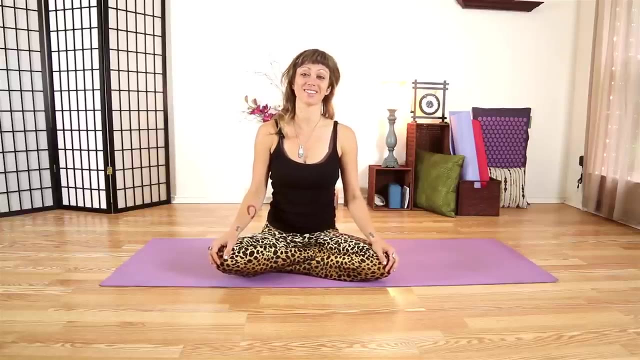 for setting aside this time to take care of you. you deserve it and nobody's going to do it for you, so I'm proud of you. thanks for being here and thanks for following along, and if you haven't already, thumbs up this video, favorite it, so you can come back. 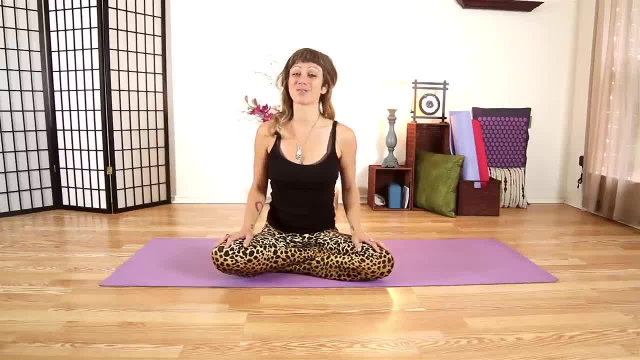 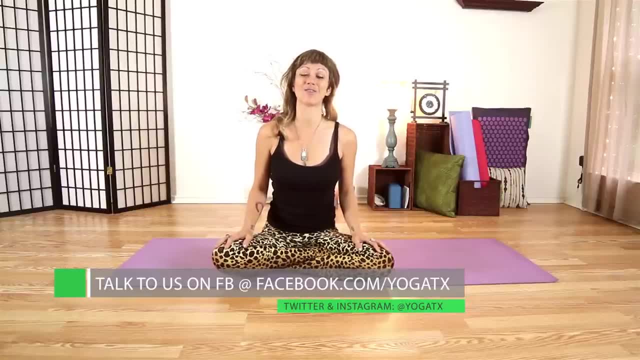 and do this practice with me again. don't forget to leave your comments below. I always love getting your feedback. let me know what else you'd like to learn, what else you want to work on. I'm here to help you improve your wealth, your health and well-being. 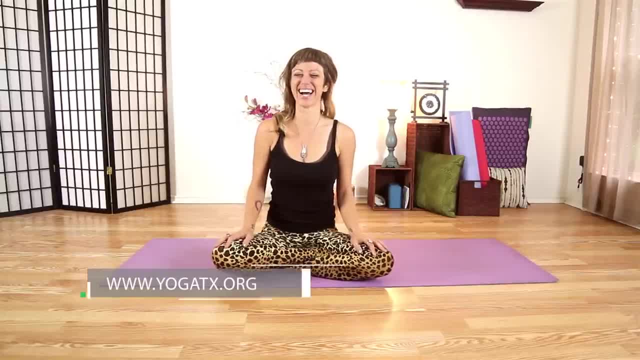 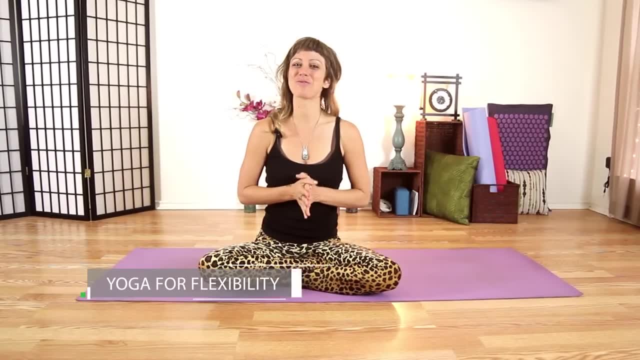 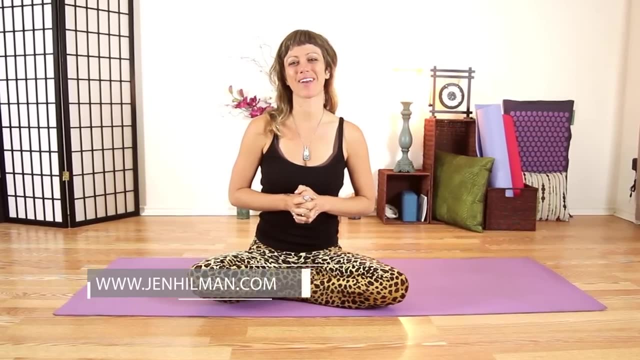 and maybe your wealth too. that'd be great. subscribe to the yoga TX so you can get our full series of yoga for flexibility, and visit my website, jenhillmancom, to keep up to date with me and all the things that I'm doing. thanks for following along.